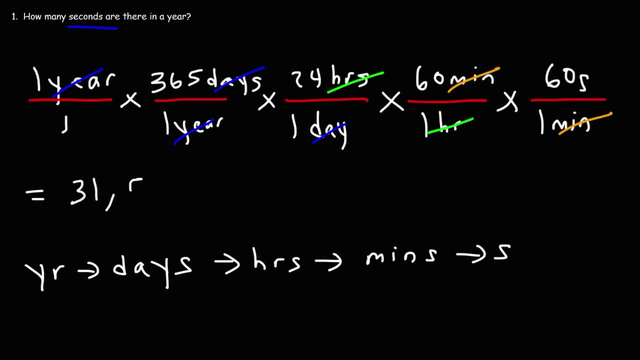 So the answer is pretty big: It's 31,536,000 seconds. So that's how many seconds are in. Now let's work on this problem. Convert 30 feet per second into miles per hour, So let's start with what we're given. That is 30 feet per second, So that's the speed. 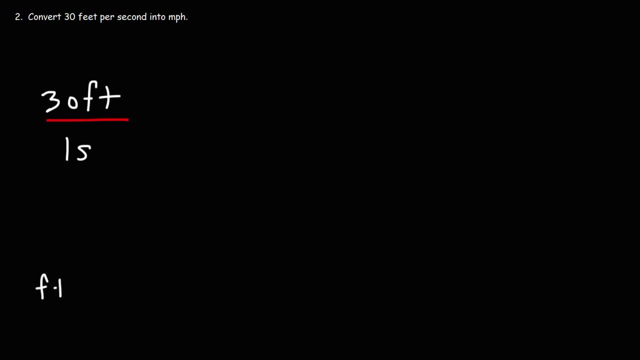 Now we need to convert to miles per hour, So we need to convert feet into miles and then eventually seconds into hours, which we know how to do. You need to know that one mile is equal to 5,280 feet, So we could put 50 to 80 feet on the bottom and then one mile on top. 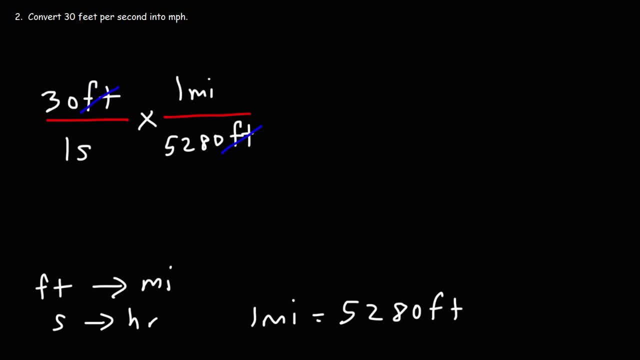 So we could cancel the unit feet, and so we have the first part of our answer: miles. Now the last thing we need to do is convert seconds into hours. Now we know that there's 60 seconds in a minute. So because we have the unit seconds on the bottom here, we're going to put 60 seconds on top so that those two units cancel. 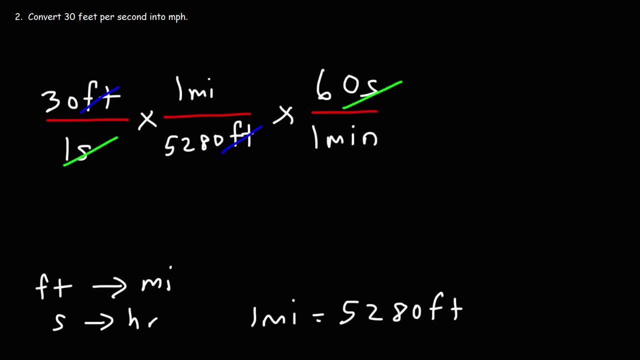 And we're going to put one minute on the bottom. Now the last thing we need to do is convert minutes to hours. So, since we have minutes on the bottom, we're going to put on the top. There's 60 minutes in one hour. 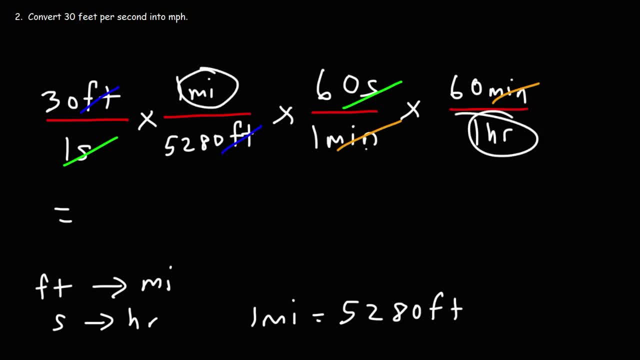 So now we have our answer And we're going to put our answer in miles per hour. So it's going to be 30 divided by 5,280.. We're dividing by this number because it's on the bottom, And then we're going to multiply by the numbers on top. 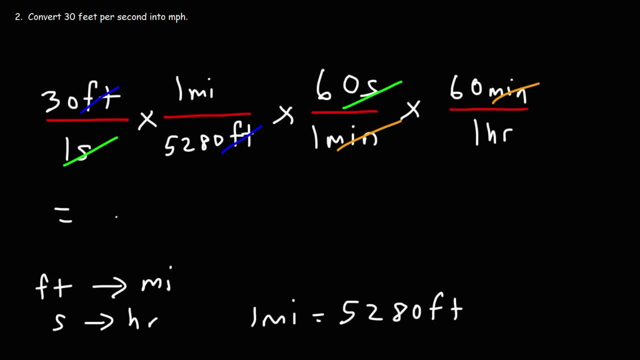 So times 60, times 60.. So it's going to be 20.45 miles per hour. So that's how you can convert Feet per second into miles per hour using dimensional analysis. Here's another problem. The ratio of boys to girls in a certain classroom is 4 to 5..